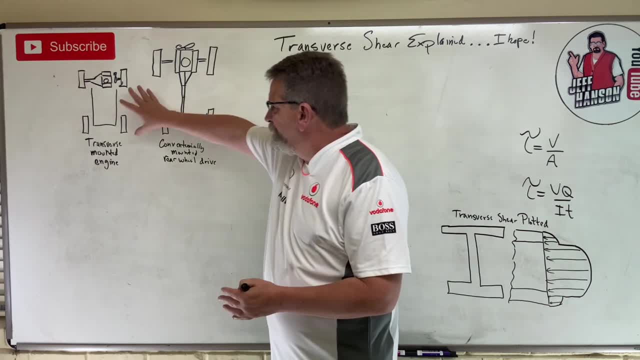 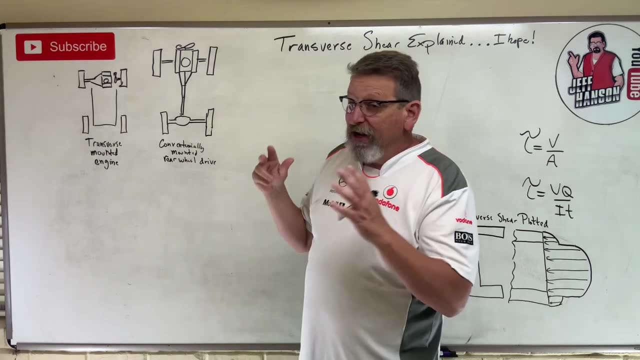 different kinds of cars. You've got your rear wheel drive car and your front wheel drive car. This is a conventional way to mount an engine so that the drive shaft is along the axis of the car. Transverse means perpendicular, or crossways, if you will right. So in a transverse mounted 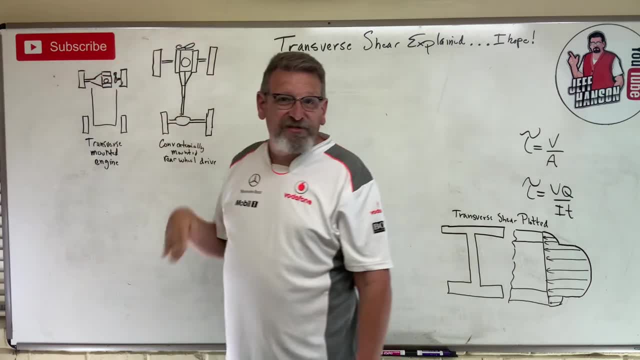 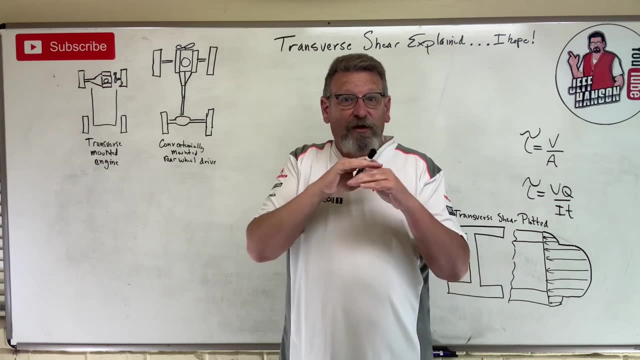 engine. instead of mounted in the conventional direction, the engine is mounted sideways, And that's how front wheel drive cars work. So that transverse word means kind of sideways. So we're thinking about shear. I'll give you an example. right, We think about shears. If I have 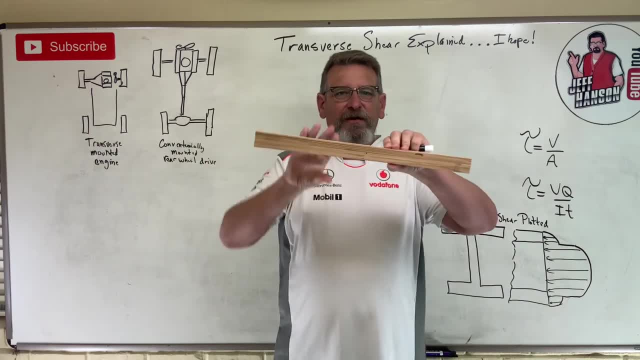 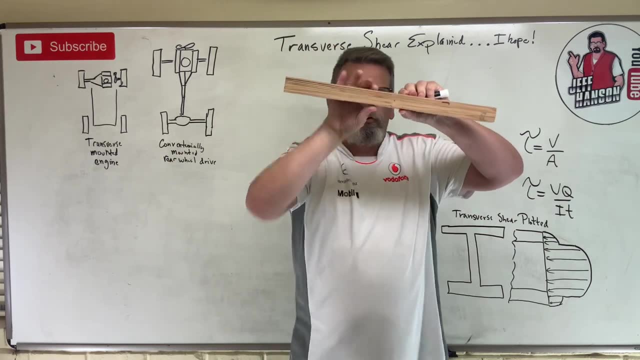 a little beam, like this guy, a little wooden beam. okay, As if I put a load on that beam, it's trying to tear it in half. right, If I push down on it, I'm trying to rip that beam in half. 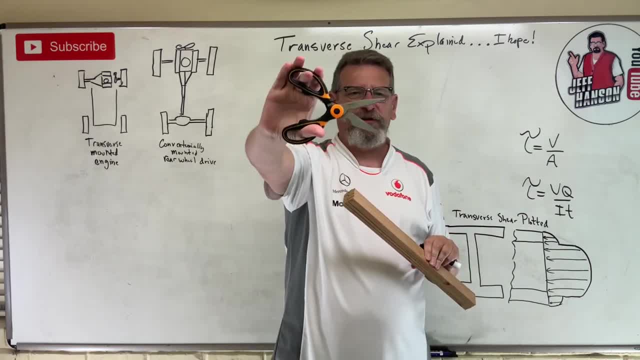 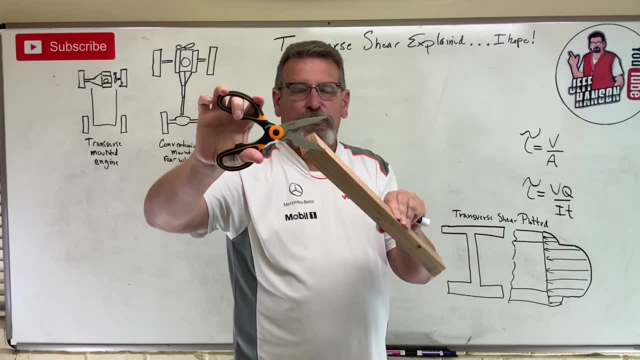 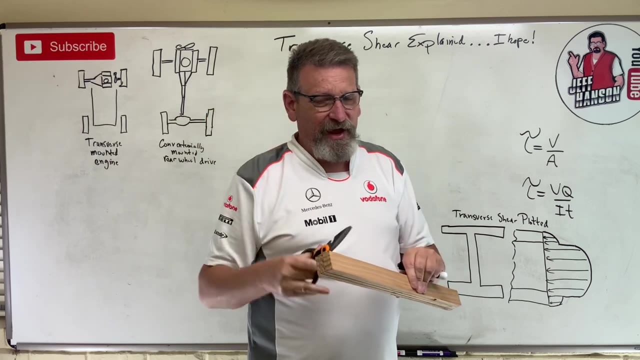 you know, That's how shears work. How do scissors work? Well, on one side- this side is pushing down on the paper, while this side is pushing up on the paper, And basically it's a controlled tear, isn't it? It just shears the material in half. 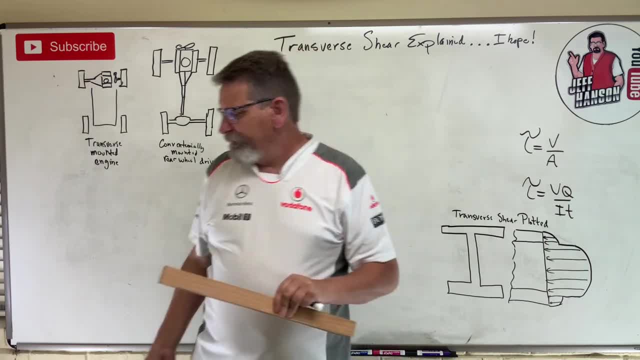 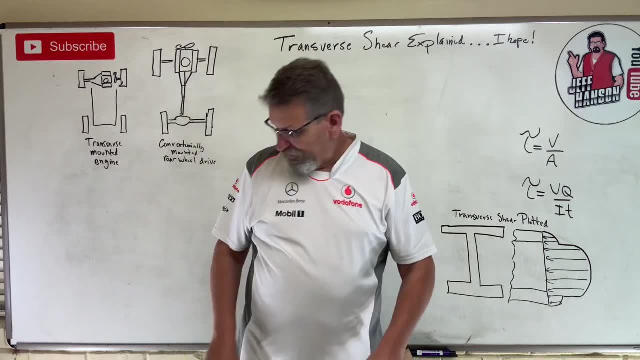 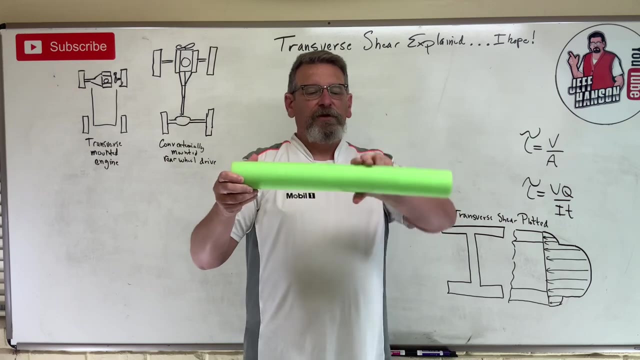 And that's what we talk about when we're talking about shear in a beam. So I think for the most part everybody kind of understood what shear stress was Like. here's one of my noodle beam. okay, So if I push down on one side and up on the other side, I get this kind of a tearing action. 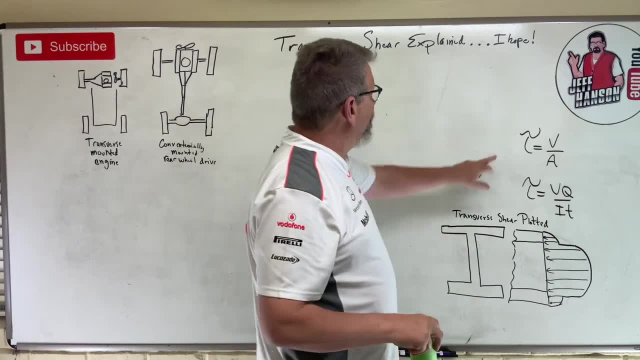 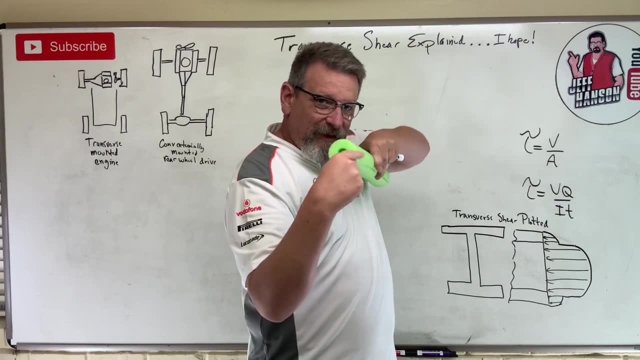 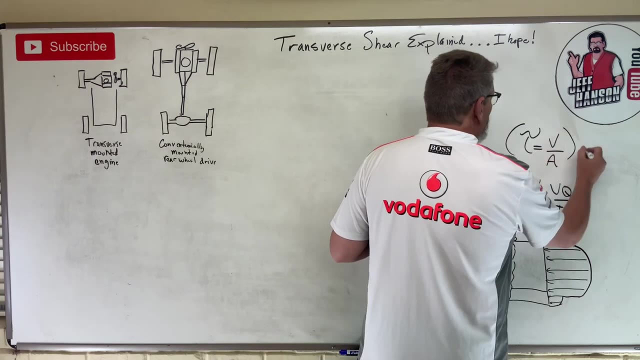 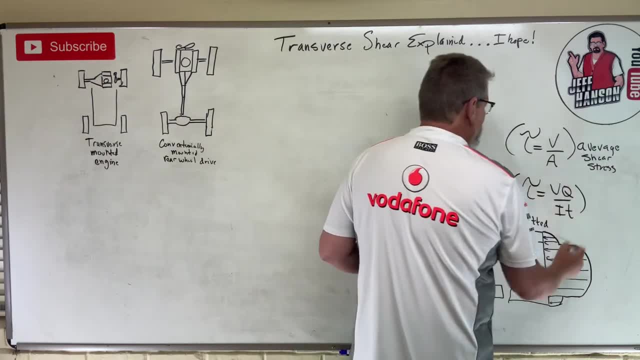 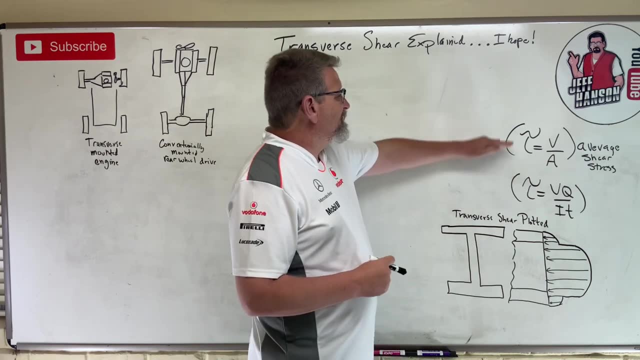 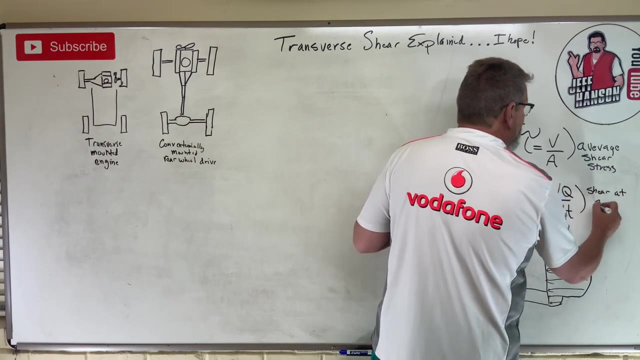 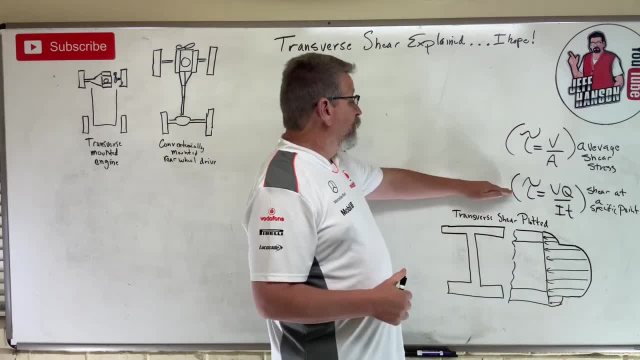 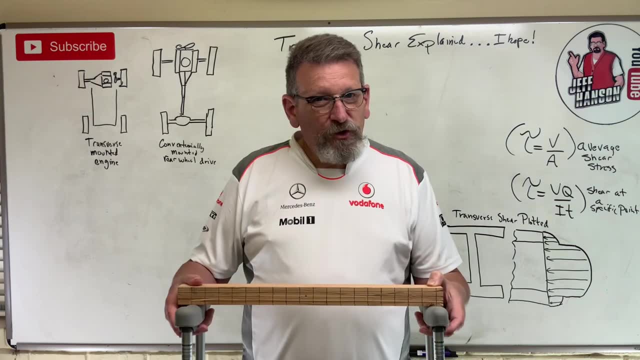 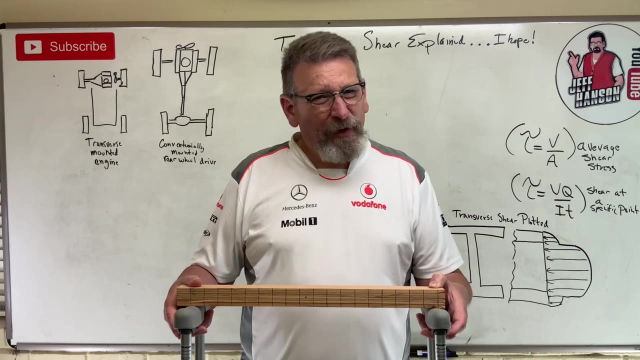 Whereas this is like average across the whole face. this will tell you the shear value at any point on the beam. Now let me give you an example of that. So I want you to imagine a beam as being made up of a whole bunch of small layers. Do you remember? we had a slinky example before. 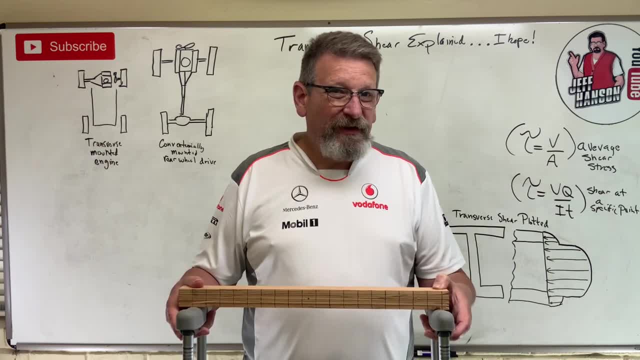 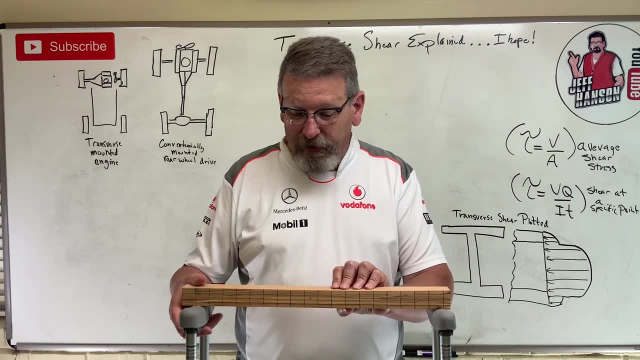 we said that when we talk about shear due to torsion, that each layer of that slinky would slide one layer relative to the next. Well, we have that same kind of configuration here. So what I've got here- I've got this all balanced- is a bunch of boards, and I've sawed it right where there's. 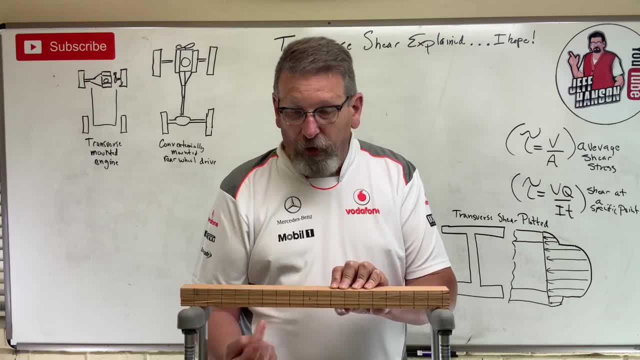 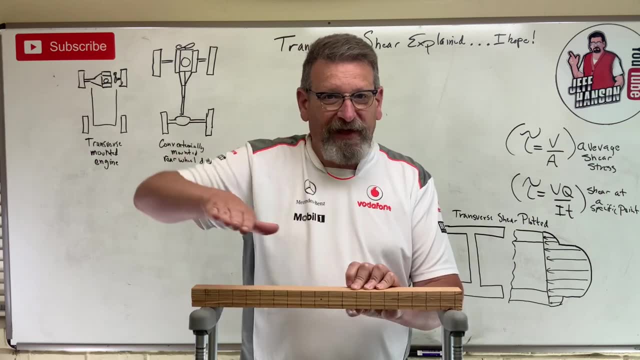 just a whole bunch of layers. Now I have come in here and I have drawn a bunch of vertical lines on this board. okay, Now, as I put a load on this board, right, you're going to see this board deflect. But what are happening to these layers as it deflects? Let me push on pretty hard here, okay. 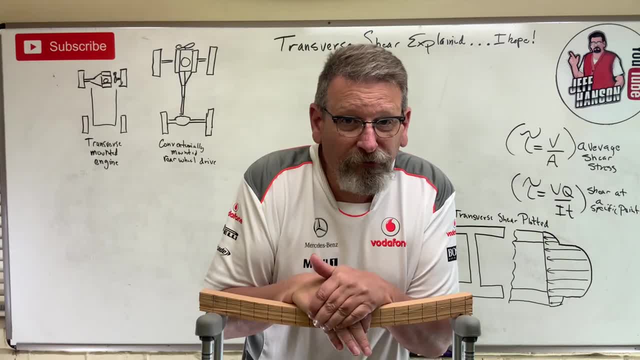 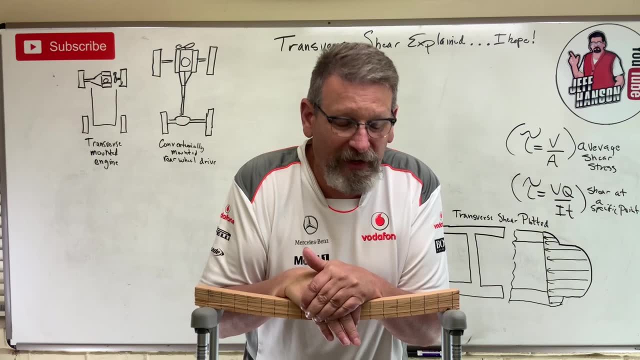 Can you look at the ends? Can you see what's going on? Are those are the lines that are straight up and down? are they still straight up and down or are they? are they? you can see where they have segmented right. Those lines are still straight up and down. 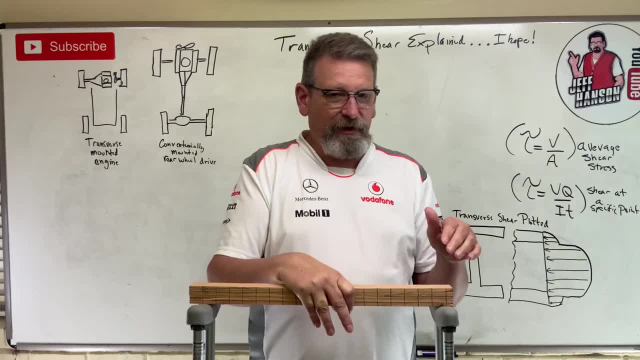 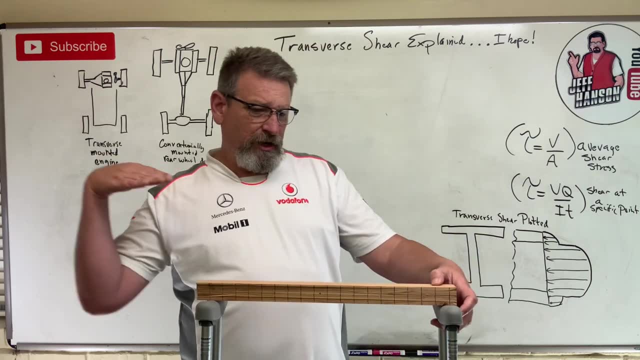 Those lines are sliding one relative to the next right Now. if I pull that back, it goes back right. So that is transverse shear. It is shearing this way on the beam, not this way in which we think right. 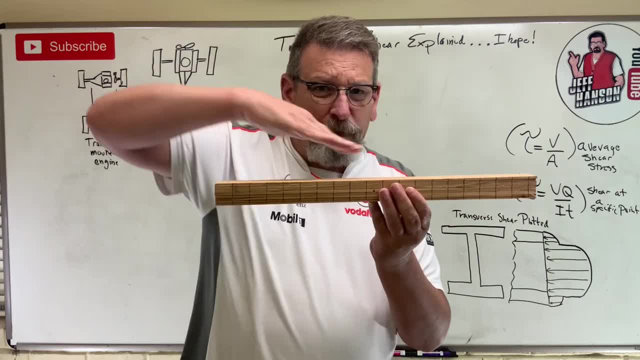 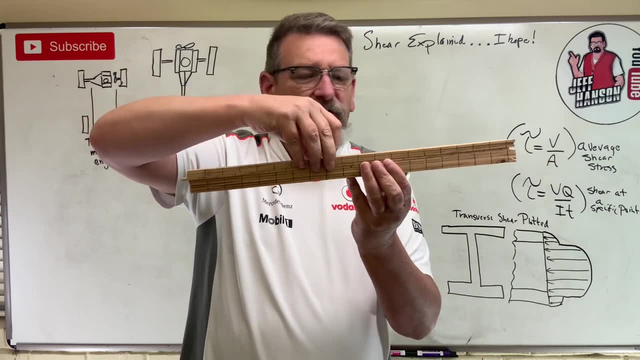 Now let's look at that right quick. So as I bend that board, that beam, right, what's happening is is these layers are sliding across each other, one relative to the next. So even if you have a beam that's not solid, right, like this direction, right? 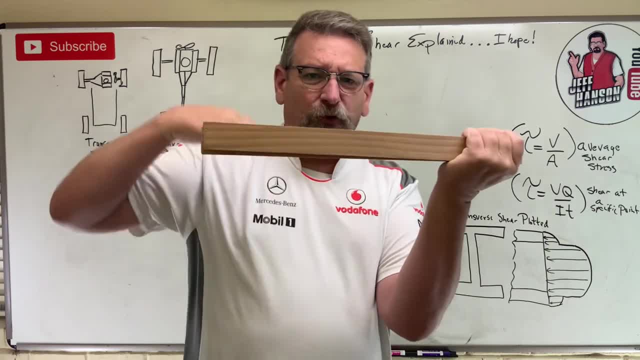 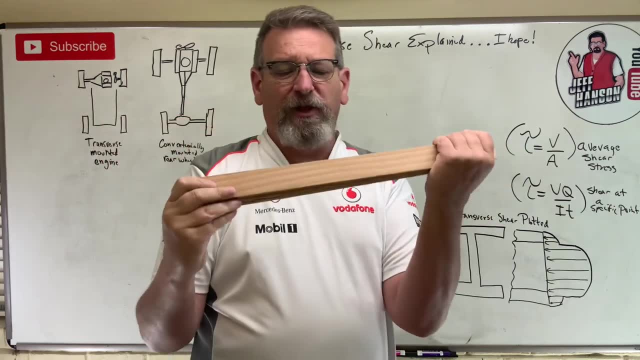 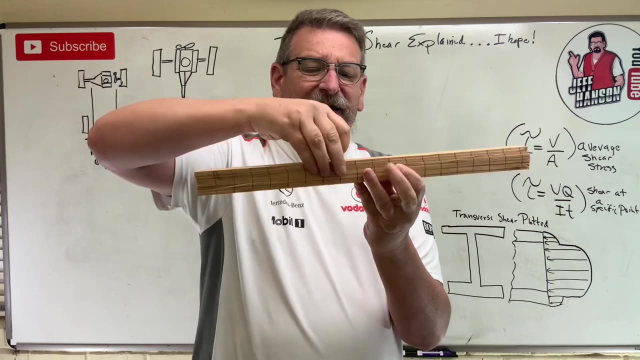 imagine, as I bend, that those layers are trying to, those fibers of the wood right are trying to slide across each other in this direction, one relative to the next right, And we can see that in the example where I just bent this right. So as I bend this, they're sliding like so okay. 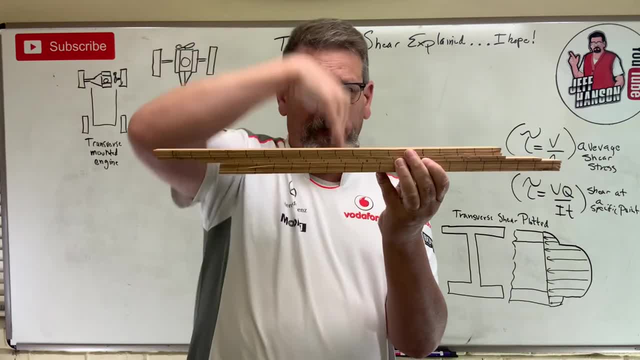 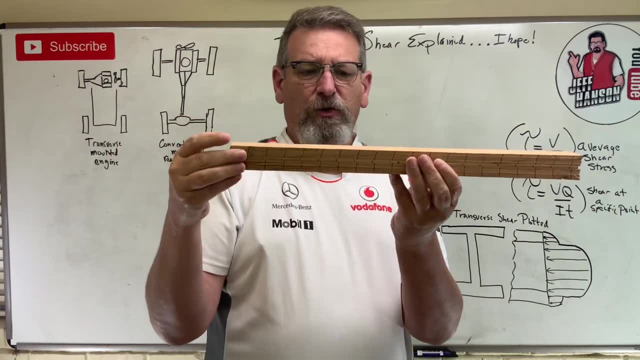 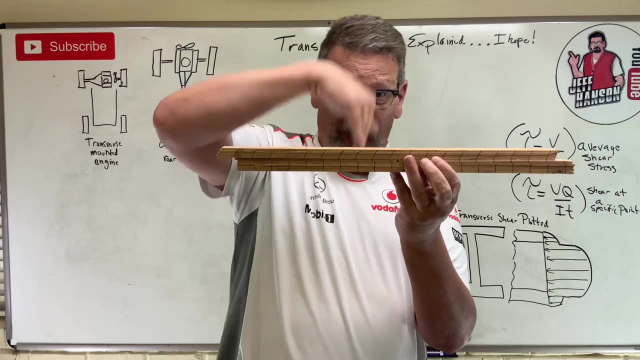 That's the transverse direction, not what we typically think of this way. So wait a minute. how does V over A, which we talked about being this way equate to now? the force is going this way. Seems like I'm adding apples and oranges here- right, an X force to a Y force or a? 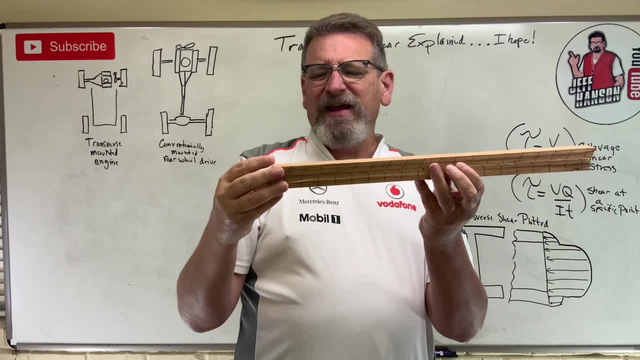 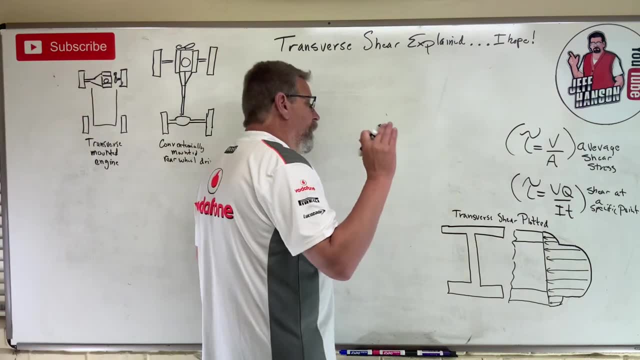 an X shear to a Y shear. That doesn't make much sense to me, okay, Let me. let me see if this makes sense to you, okay, Okay. so the first thing let's just talk about. what are the components in? 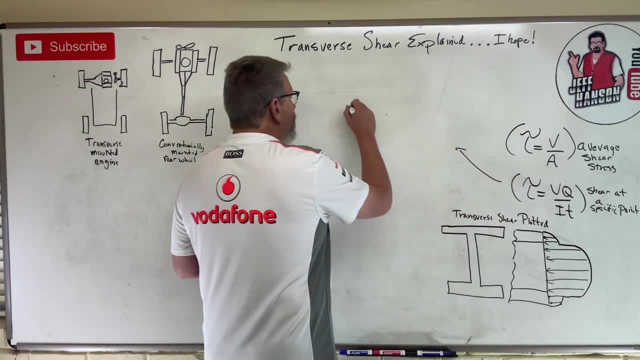 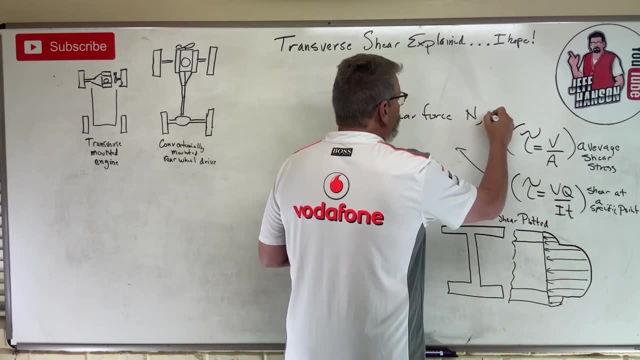 this equation here, okay. So what are those components? Well, you've got V, which is the shear force, okay, And that's going to be in something like newtons or pounds, or kilonewtons or kips. 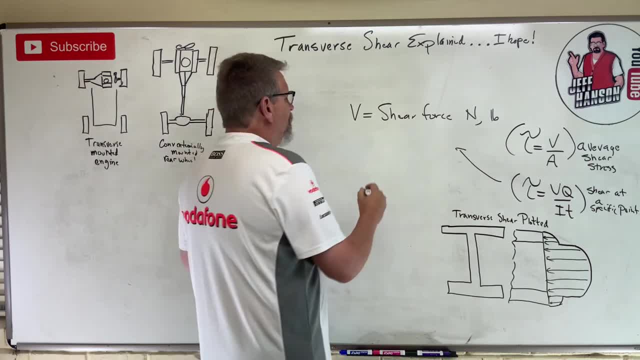 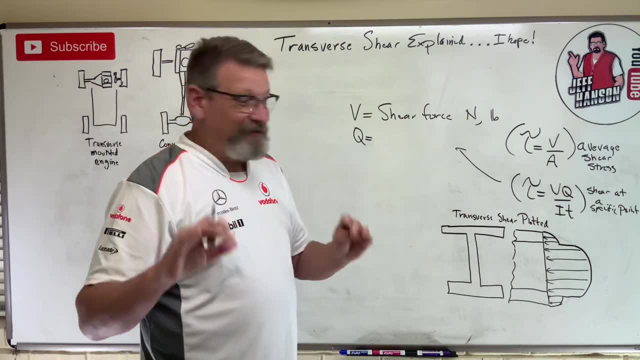 or something like that. right, It's a force. okay, Then you've got Q. And if you don't get Q, go back and watch my video that says what the heck is Q? right, I think that's the name of the. 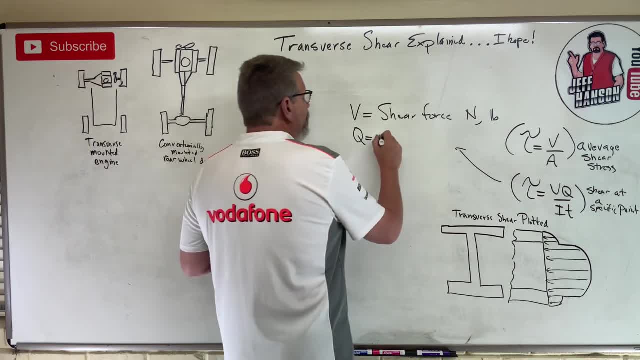 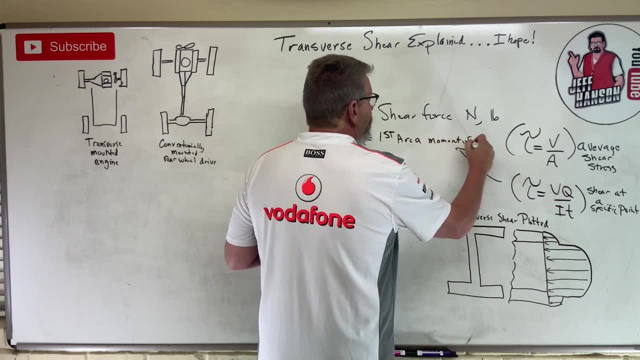 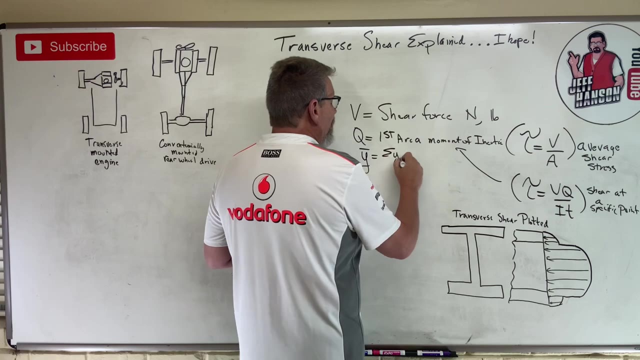 video right And I'll explain to you what Q is. It's the first area moment of inertia, okay? And Q is: remember this guy: Y bar is equal to the sum of the Y A's divided by the sum of the A's You. 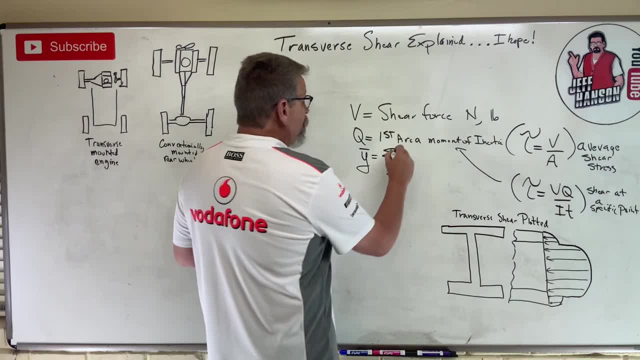 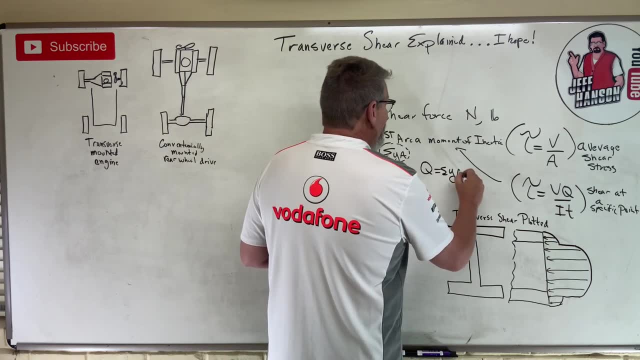 remember that from statics the old Centroid equation Q is just this up here. okay, It's the top half of the Centroid equation, So Q equals the sum of the Y times A's. Again, if you don't get that, go watch that video and explain what that is, because it's a very 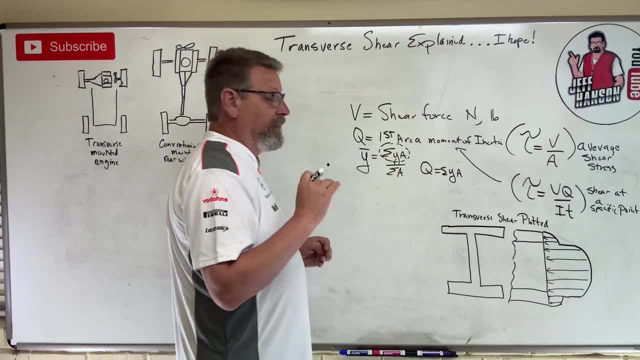 challenging concept for students to get. We're going to use Q here a lot, And then, of course, we know what I is. I is the X force. So let's go back here and we're going to use Q And then of. 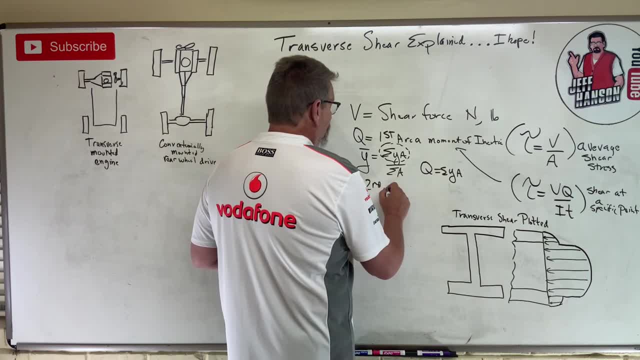 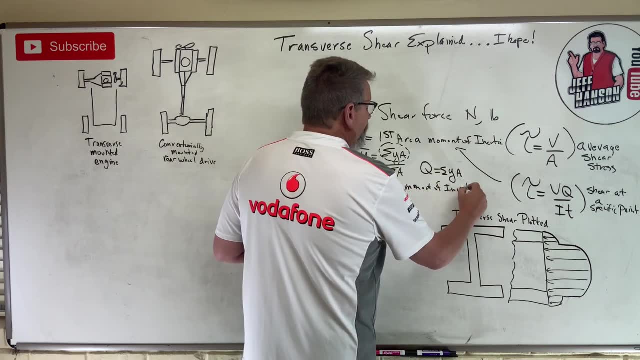 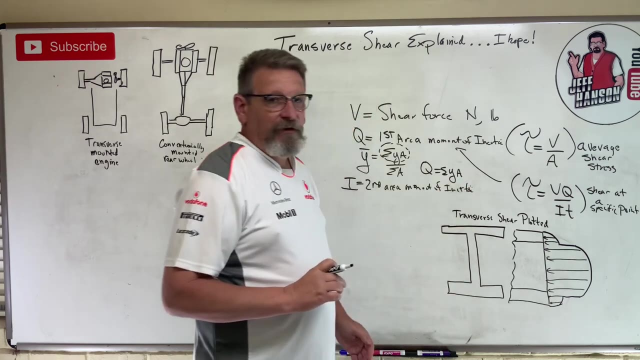 course we know what I is. I is the Y force. remember this guy and this method for the centroid equation. I is the second area, moment of inertia. okay, And that is a geometric property of the cross-section of a beam that tells its resistance to bending right. 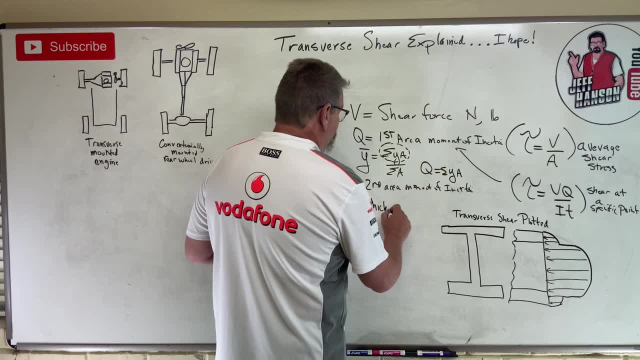 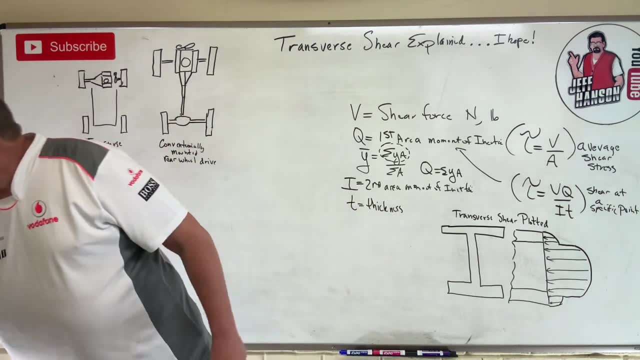 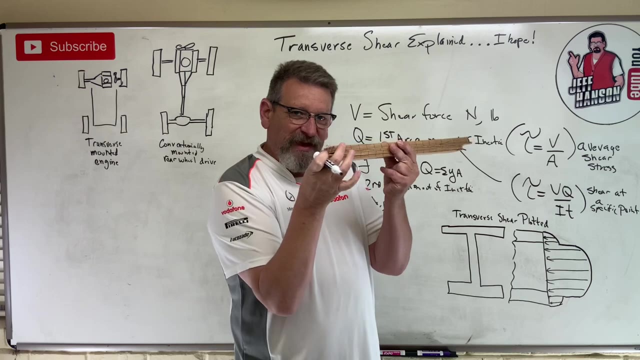 Whereas the last one, T, is just the thickness of the beam. So always think about the thickness of the beam as the amount that I would have to tear through, right? So if I'm going to transverse here this way, right, what thickness of the beam am I going to have to tear through to make those layers slide? 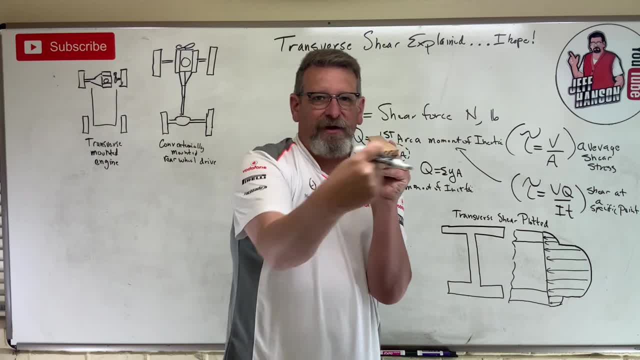 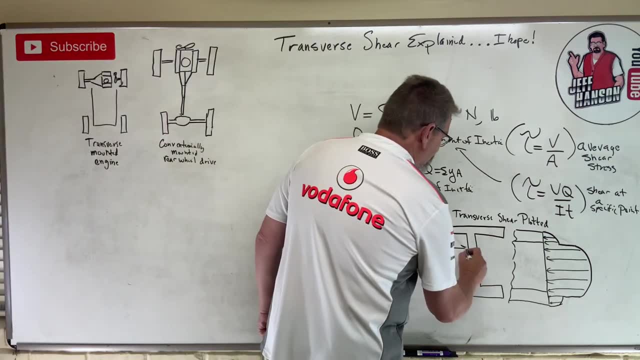 Well, in this case, the thickness would be this width right here. right, That would be the thickness. okay, In the case of our I-beam here, right, this is the thickness here. Well, this would be the thickness. 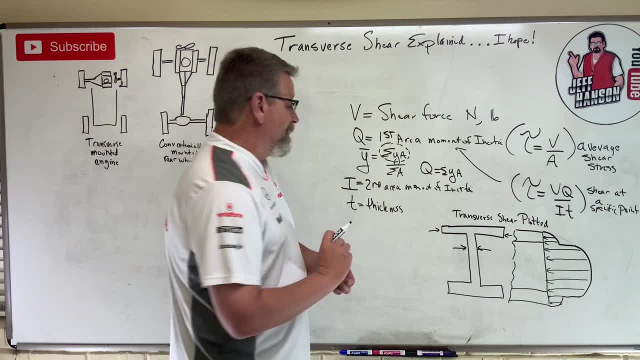 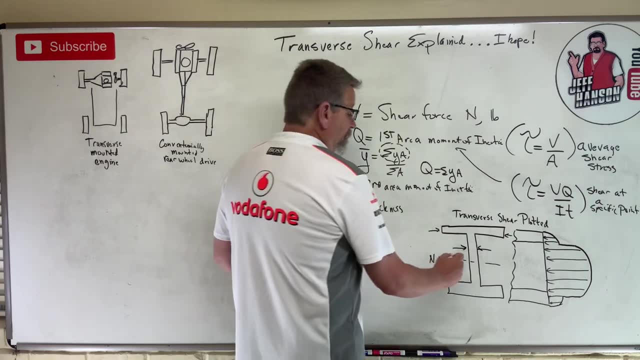 This would be the thickness up here, wouldn't it right? So it depends on which point I'm asking you to find it at. So let's say: this is our neutral axis. okay, Then remember what this is called. This is called the web. 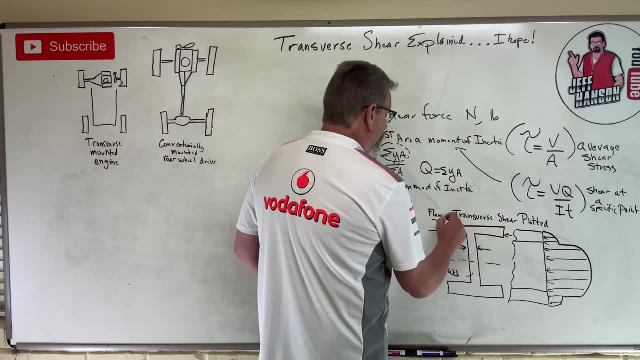 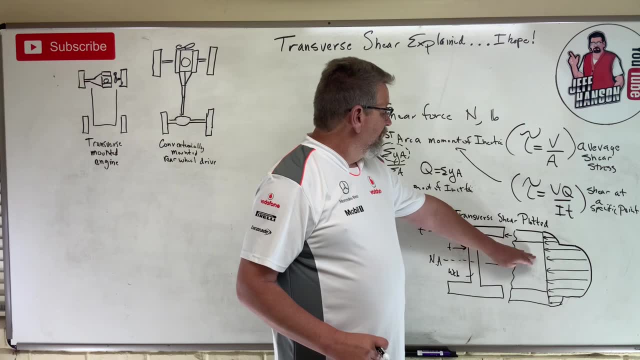 This is called the flange. okay, This would be T up here. This would be T down there. Now, this is over here. what I've got is a transverse shear stress plotted right. So this is here's the cross-section of the beam. 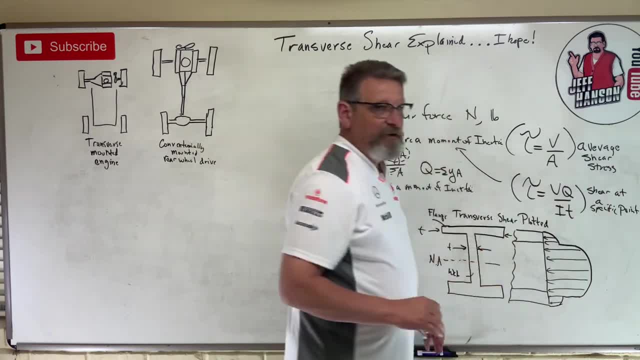 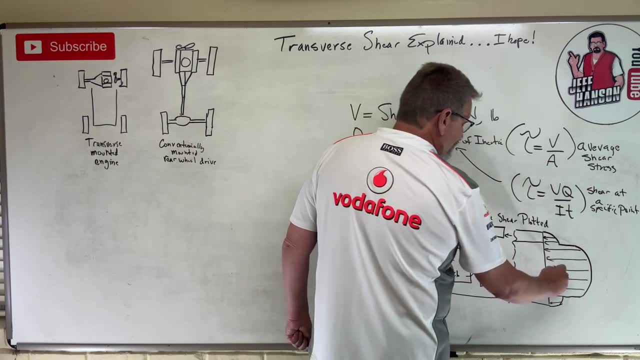 This is going to be like looking at the end of the beam. if the beam was going this way, right? So what's going on over here? Well, look at this As in the middle, right at the neutral axis, right here, that's where the shear stress is greatest. 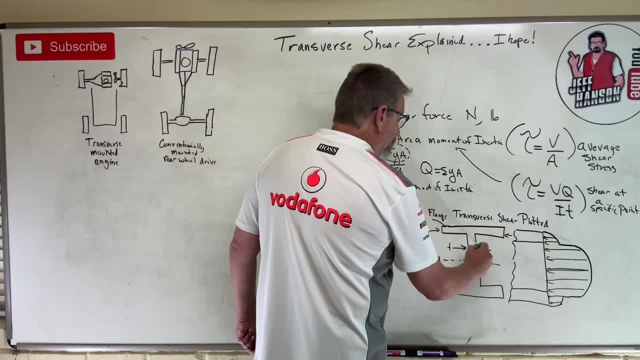 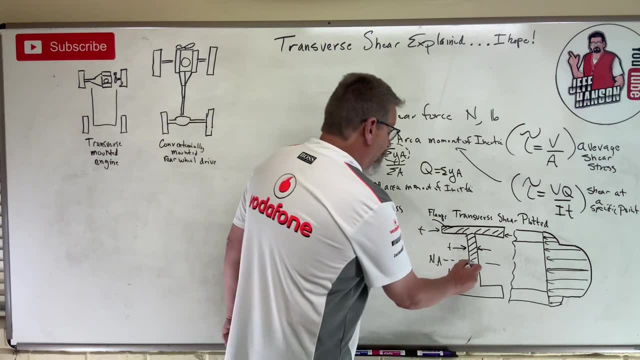 Why is it greatest? Because Q would be all of this up here. right, It's Y times A above the point of interest. So if the point of interest is here, on the neutral axis, Q would be as big as it can be. 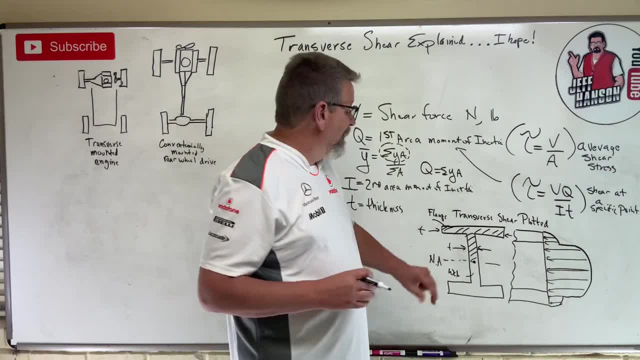 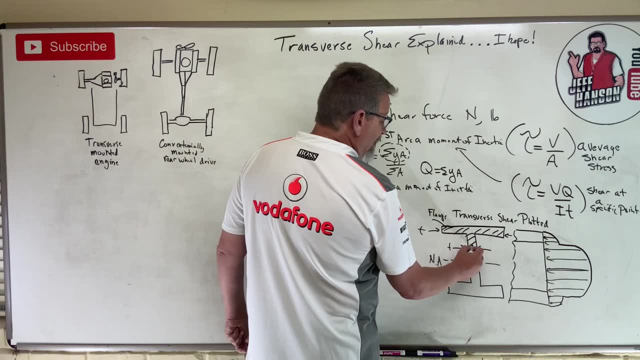 Right, Q is always as big as it can possibly be when you're on the neutral axis. okay, As I go up on the part, right, if I'm here right? well, now Q is only this top part up here, right. 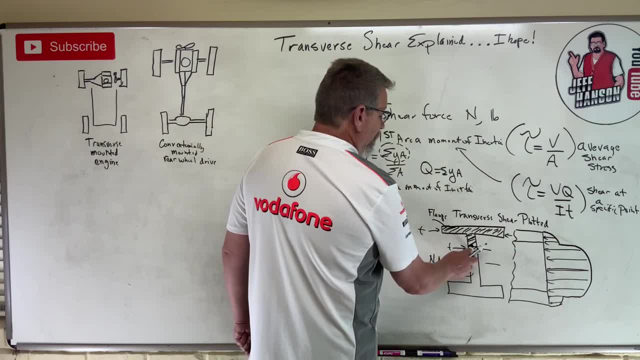 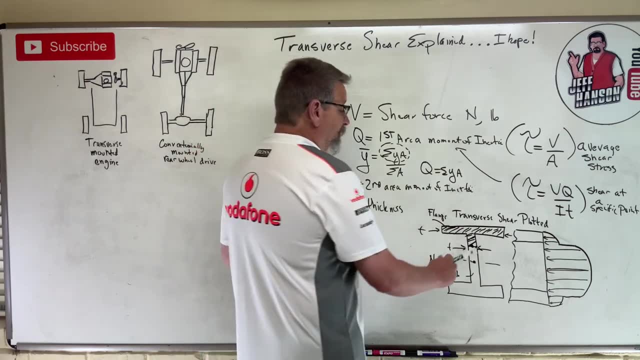 So Q just got a little smaller. It's not this bit down here, right? So as Q gets smaller, the shear gets smaller. okay, Now what happens when I go right here, when I get to this part here where the web meets the flange? 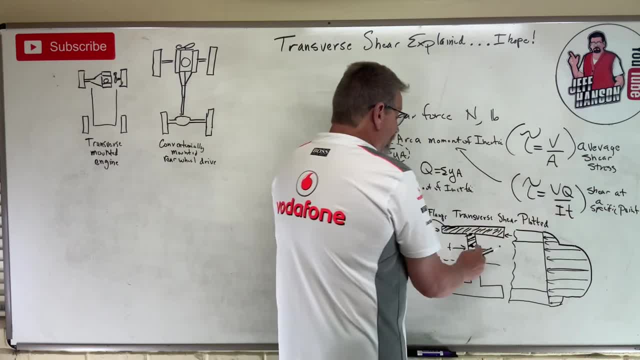 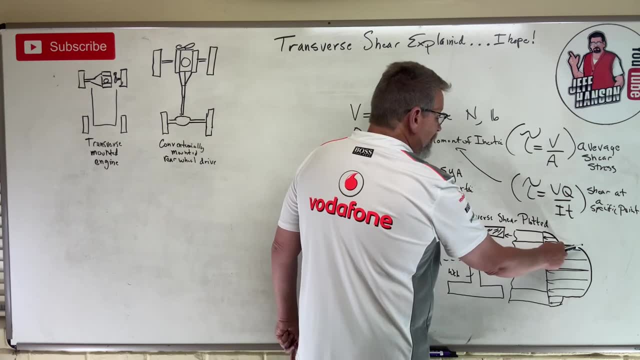 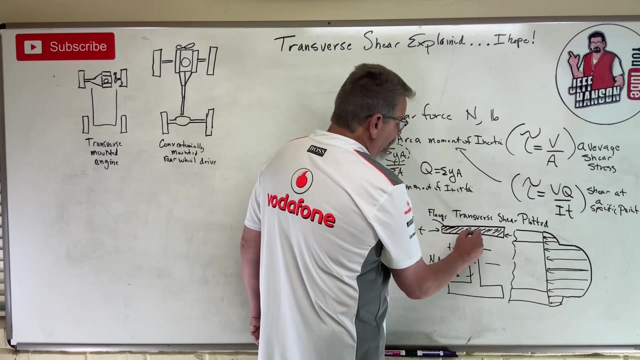 Well, what happens to T right here? I jump from a small thickness wham to a big thickness right, And so you get this discontinuity whoop, and then the stress is very small. Now, the closer I get to the outside of the part right as I get closer and closer to the outside of the part, guess what? 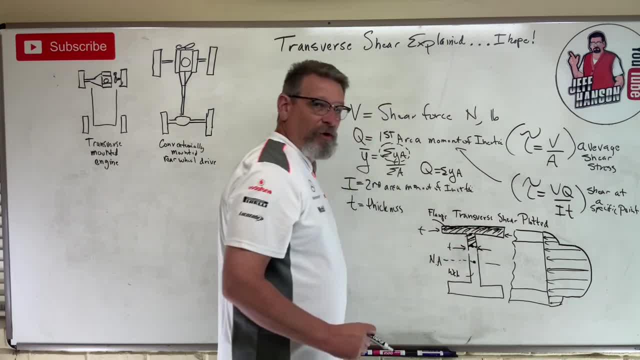 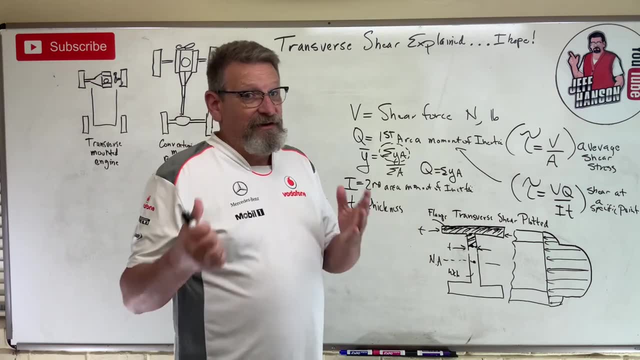 Q is getting smaller and smaller and smaller until I get to the outside of the part. Then Q is zero And transverse shear consequently is zero And transverse shear consequently is zero And transverse shear is zero. Now let me just explain to you how I think of transverse shear. okay, 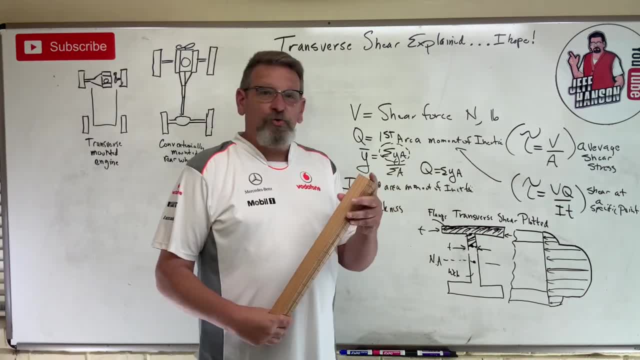 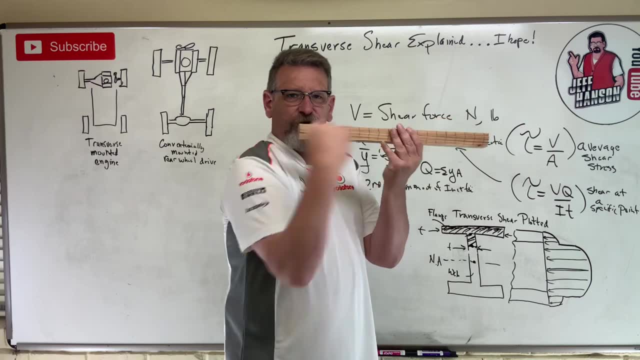 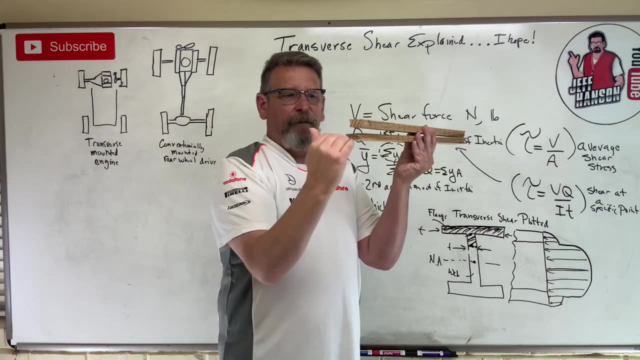 I think of it in terms of Newton's third law: right To every action there's an equal and opposite reaction. So this thing wants to tear along this transverse direction. right Here in the middle, right in the middle, I have the most material above me to resist that tearing right. 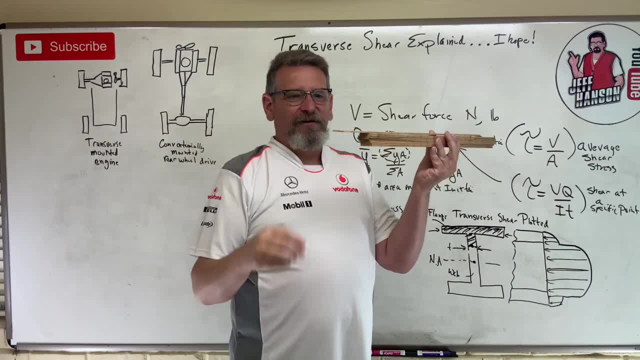 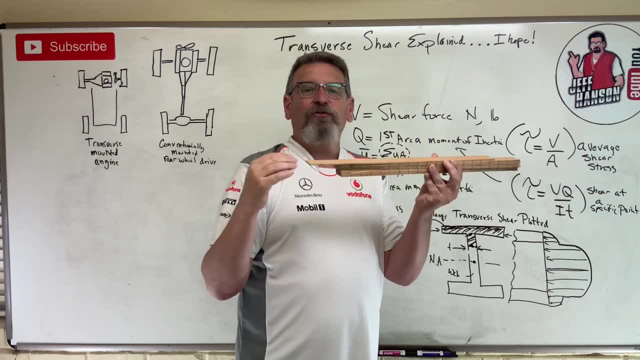 And as I get closer and closer to the outside. now I only have this much material up here to resist that tearing right. I don't have anybody to oppose me When I get to the very top. how much material is above that to oppose me? 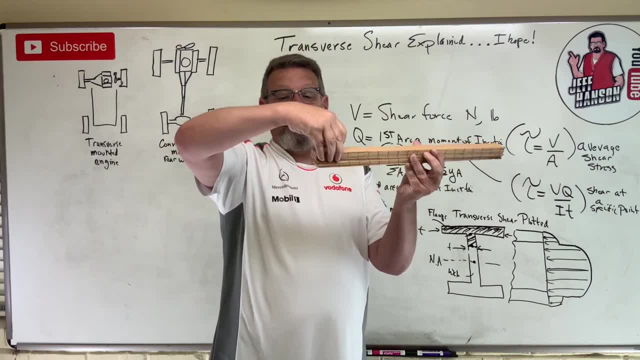 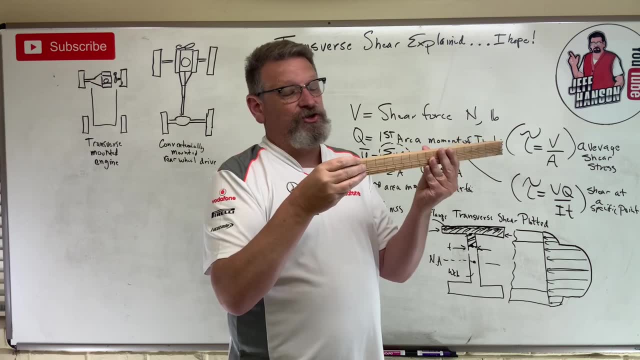 Zero right. So in the middle I have the most structure to oppose that shearing And that's why the shear stress is highest there. When I get to the outside, there's nobody to oppose me And so the shear stress goes to zero on the outside of the part. 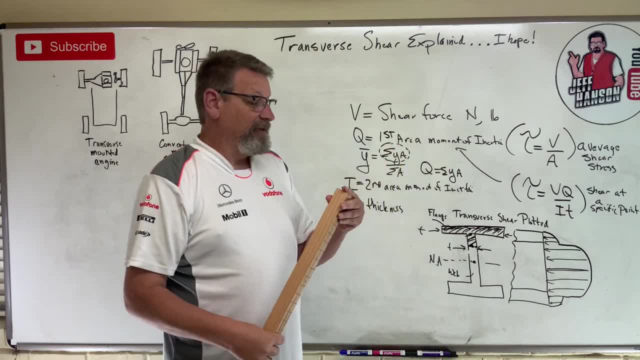 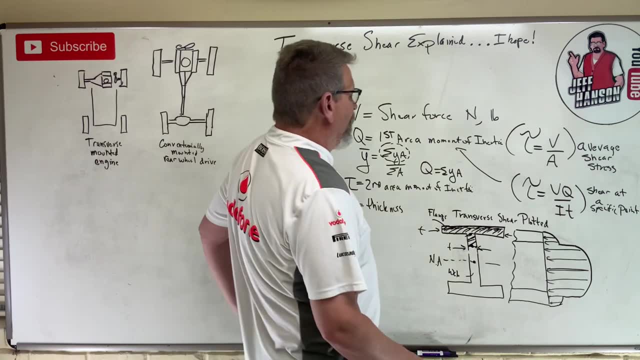 That's kind of the way I think of that, And I think that makes a lot of sense. Okay, now let's go. And then one more thing here, and that is that V over A is the average. So what I can do is, with this equation I can calculate the shear stress anywhere. 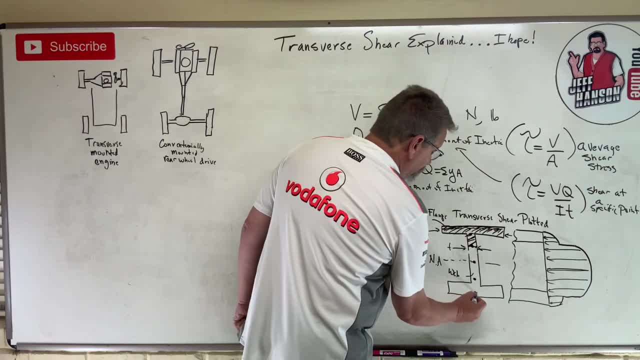 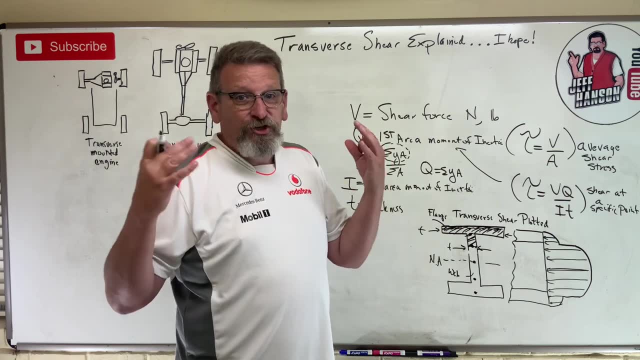 You want to know what it is right there, I'll tell you. You want to know what it is right there? I'll tell you. Why is that important to me As an engineer? if I'm designing something to support a load, what am I concerned with? 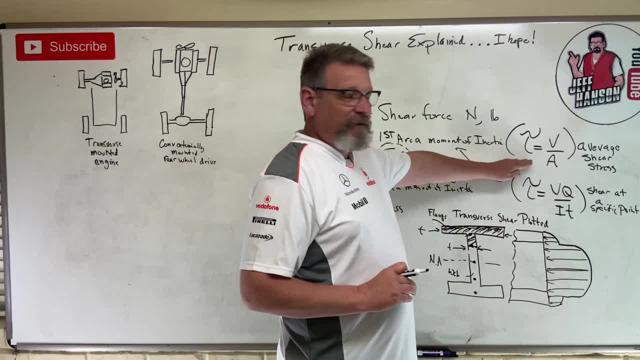 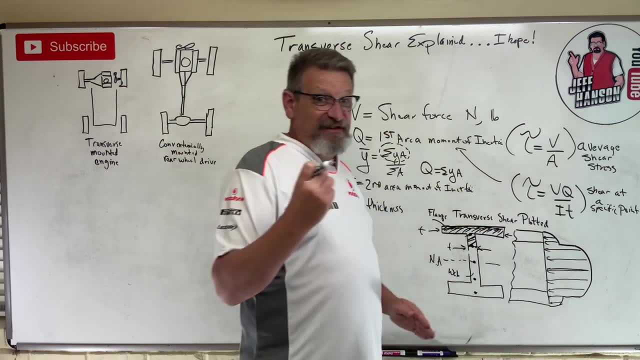 Am I concerned with the average? Am I concerned with the average shear stress? Or am I concerned with where does that absolute maximum shear stress? What is that? Because that's the thing I don't want: to fail right, I want it designed for that max. 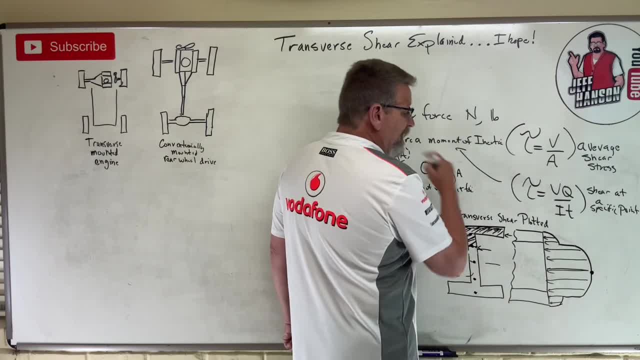 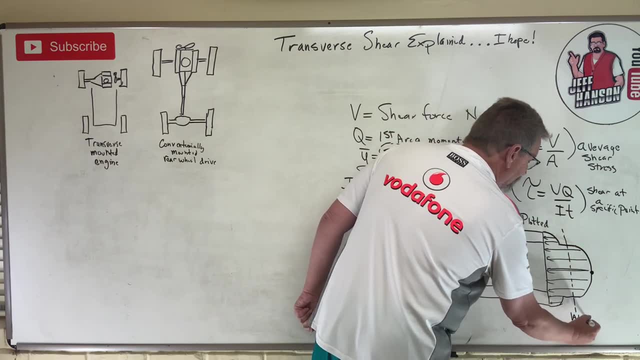 So that max is maybe here, right. So, whereas if I add all of these little arrows together, right, maybe I get like an average here. Okay, there's maybe my average shear stress, okay. Yeah, So I can do a little quick estimates and that kind of thing. 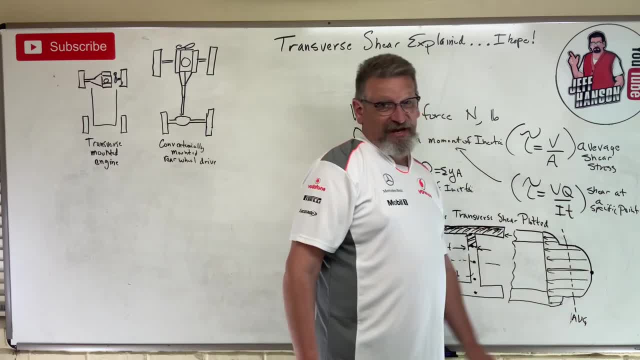 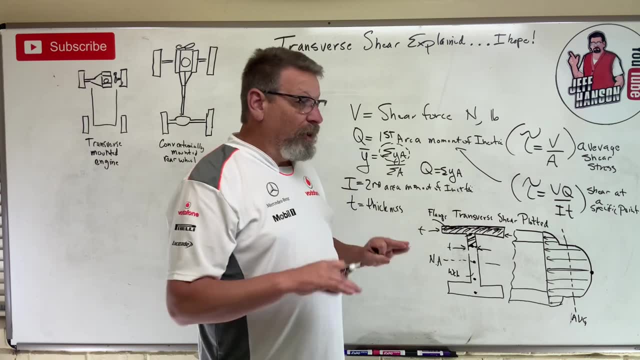 But as an engineer, I want it designed for that worst case, don't I Now for 99% of beams out there? the worst case, shear stress is always going to happen at the neutral axis, because that's where Q is the biggest. 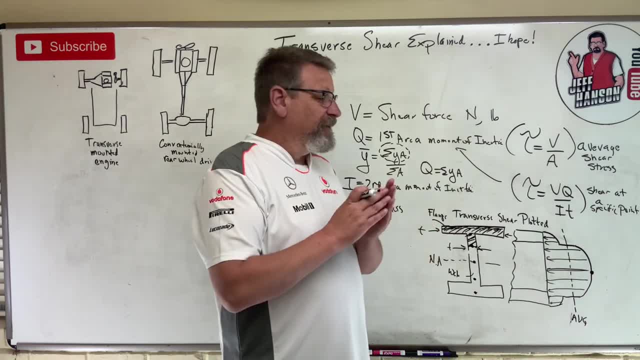 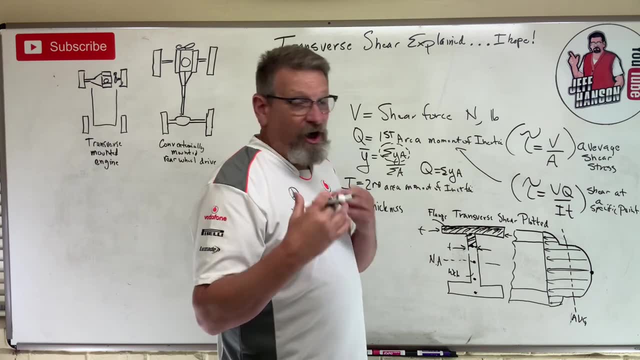 Now there are some very weird beams out there where the thickness varies. It's small here and it's big in the middle and it would flip and then the neutral axis is not where the maximum will be. But that's a very strange beam and it's a very obscure case for this. 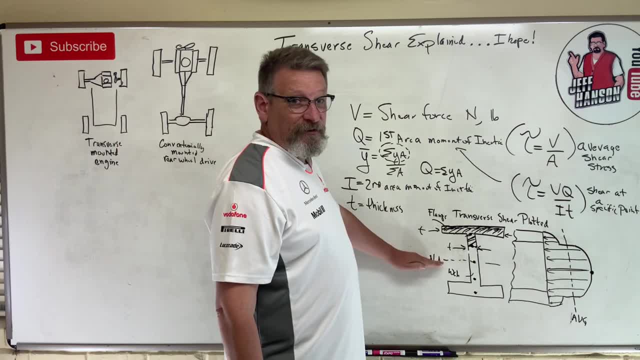 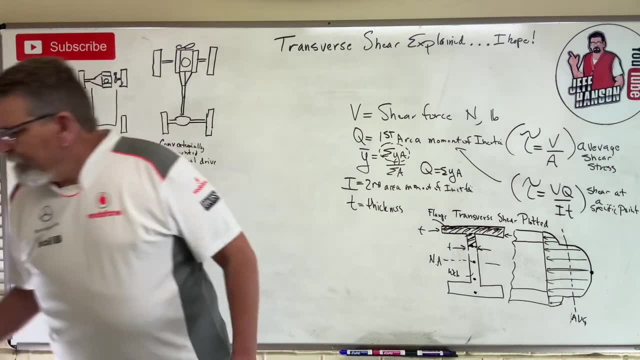 99% of the time, maximum shear stress happens at the neutral axis. okay, All right. so one more note before we wrap this video up, and that is this. okay, I know what you're thinking, Dr Hanson. wait a minute. 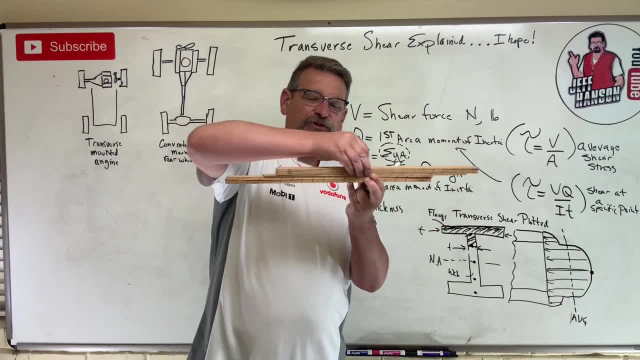 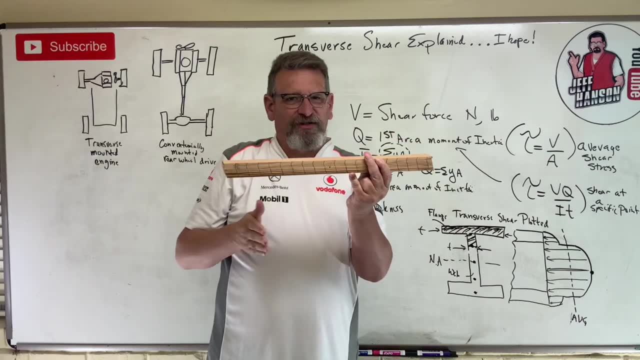 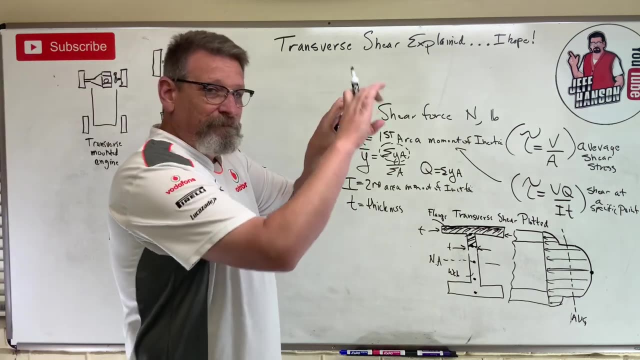 I still don't understand how a shear in this direction transverse equals a shear in this direction across the face of the material. Okay, Let's see if this clears it up. okay, Let's say that on that, where those two beams are shearing in half right. 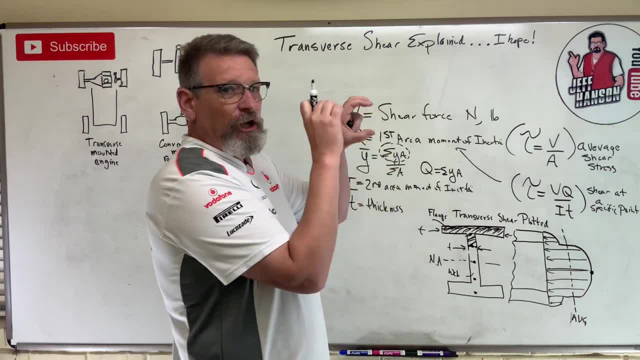 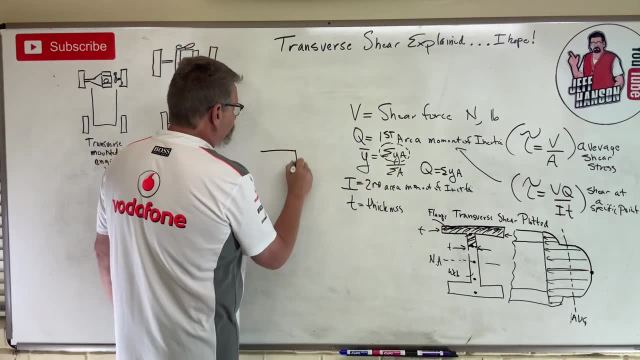 Where these two beams are shearing in half. I looked at a little bitty, tiny piece of material right on that shearing surface. okay, So maybe here he is. okay, There's that little piece of material. okay, that's getting sheared. 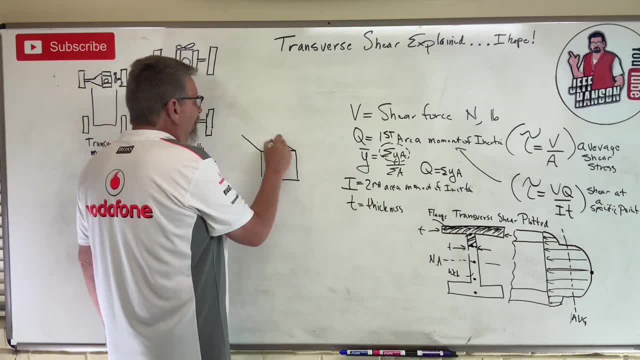 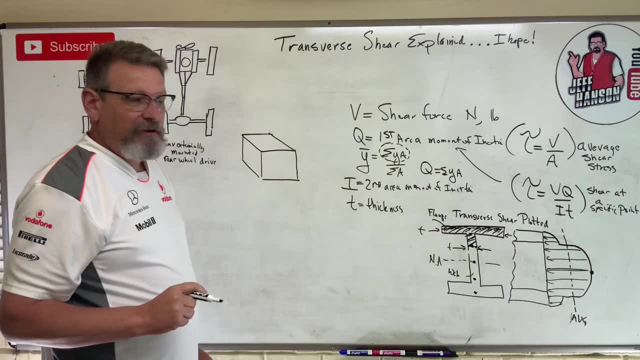 Now, you know this, don't you? You know that that little. there's no such thing as a 2D piece of material. It's a little piece of material, It's a little piece of 3D. It's a little volume, isn't it okay? 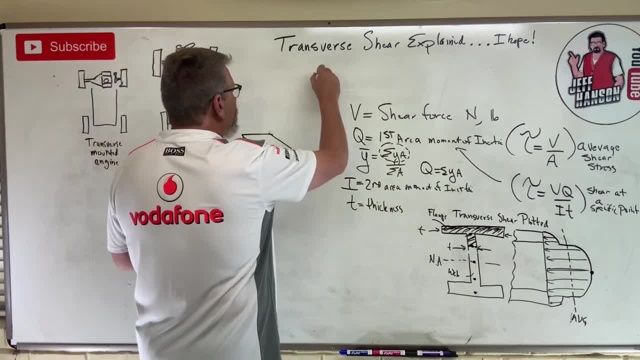 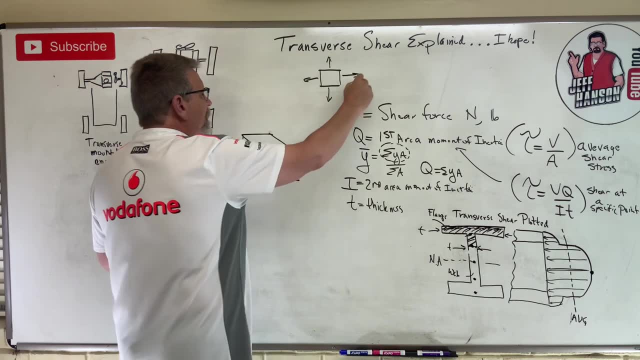 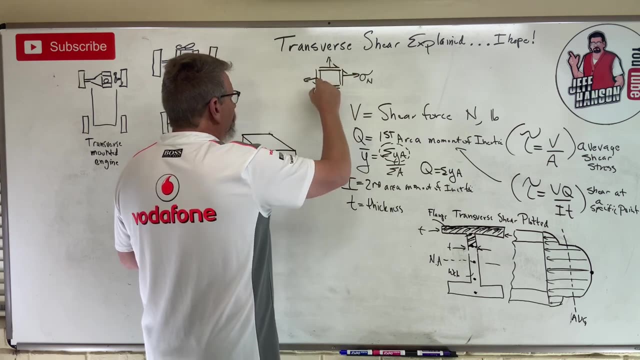 So imagine this: Whenever we sketch, whenever we sketch our stress elements, okay, what do we do? We do this number here, right? We say, hey, this is normal stress, okay, normal. And then here are those shear stresses, okay. 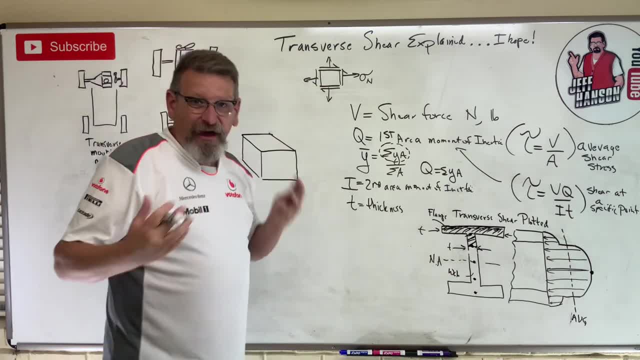 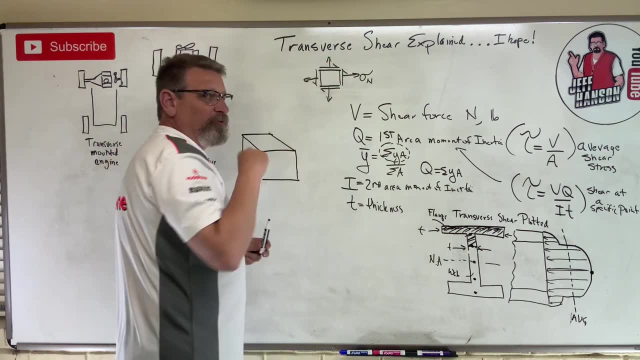 Why do the shear stresses go to the corners and meet each other? Well, they have to because of because of their reaction: Equivalent opposite reaction. Otherwise, if they didn't, these little stress elements would be spinning, wouldn't they right? 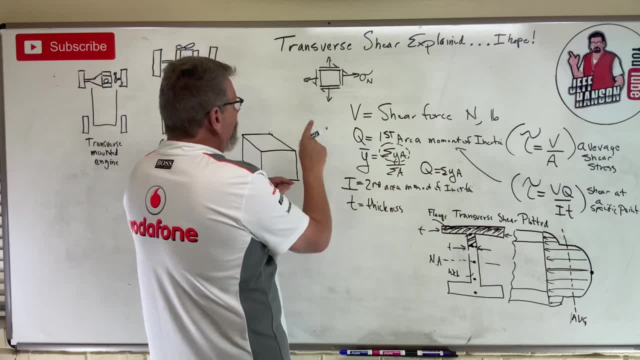 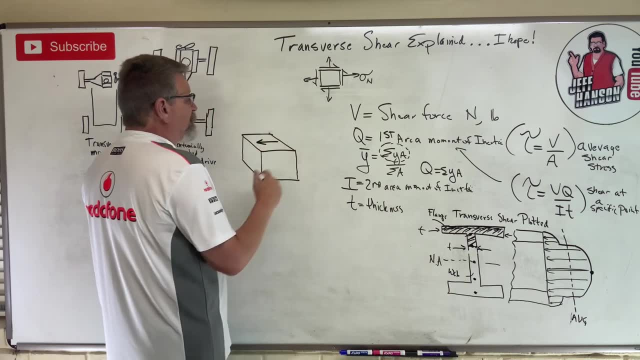 This one. you know, if I pull on you that way, somebody has to pull on me that way. If I push up, then somebody has to pull down, right. So let's just say that I had this, I had transverse shear in this direction.